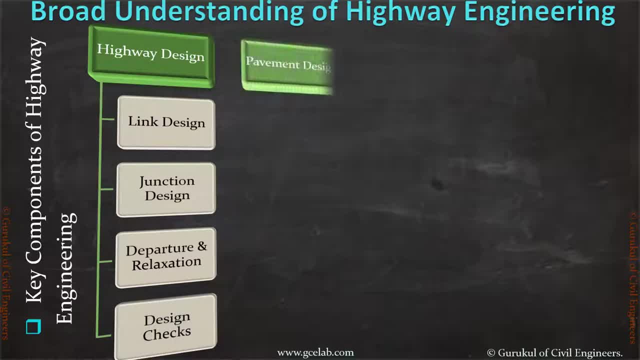 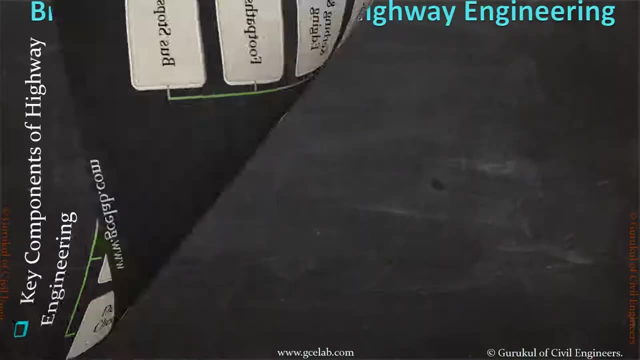 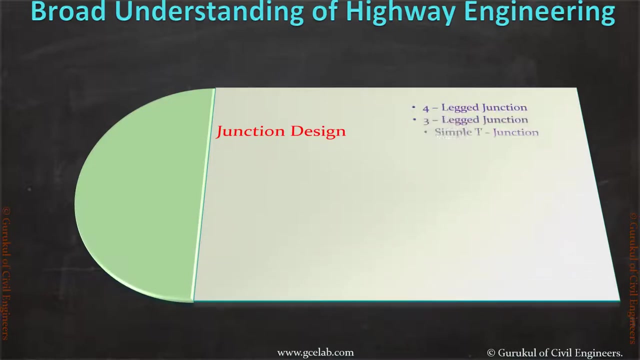 In pavement design. we will cover Cover full-depth pavement construction and overlay inlay treatment. We will also cover standard details and highway quantities. We will discuss junction design of four-legged junction, three-legged junction and T-junctions. We will also cover grade-separated junction such as: 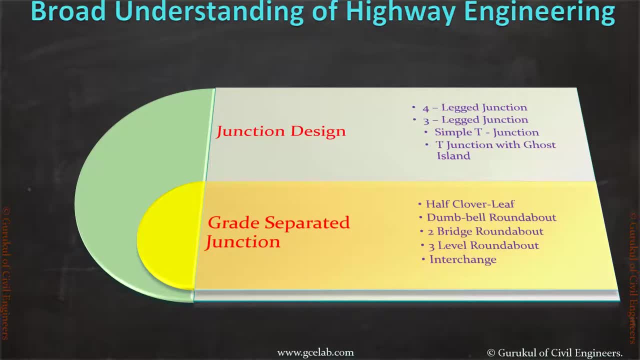 We will also cover grade-separated junction such as half clover leaf, front Geiger's, large젠ge's and large Kepler channels. We will also cover full-depth pavement construction and overlay inlay treatment leaf, dumbbell, roundabout, tube, bridge roundabout, etc. 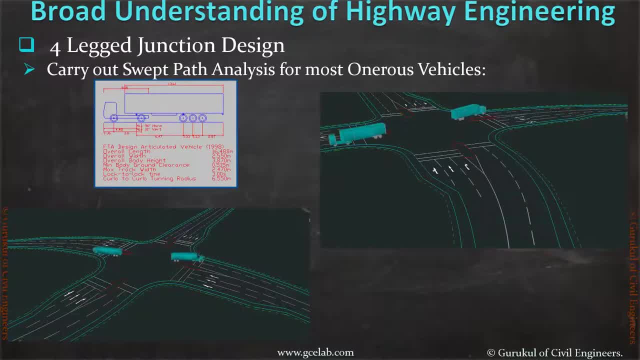 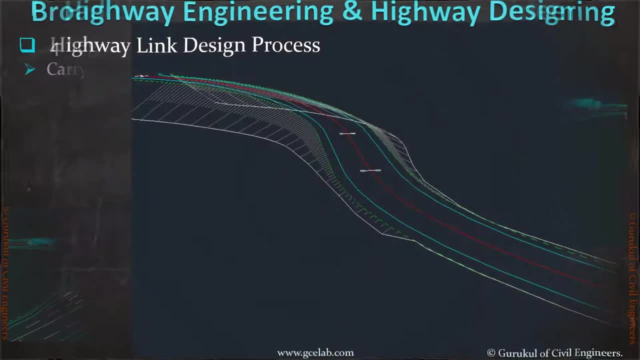 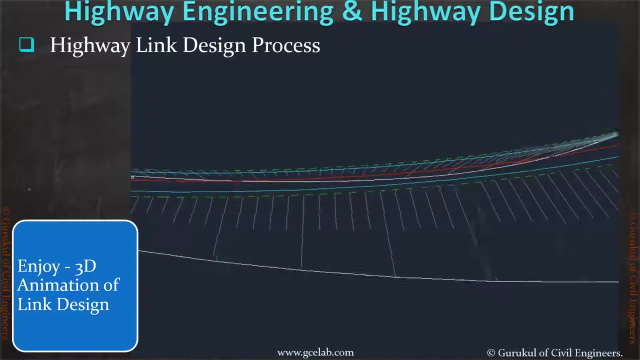 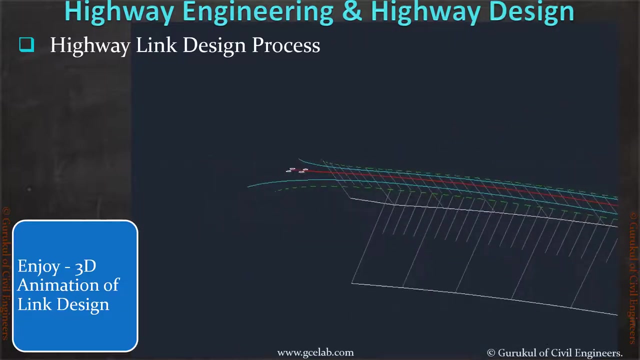 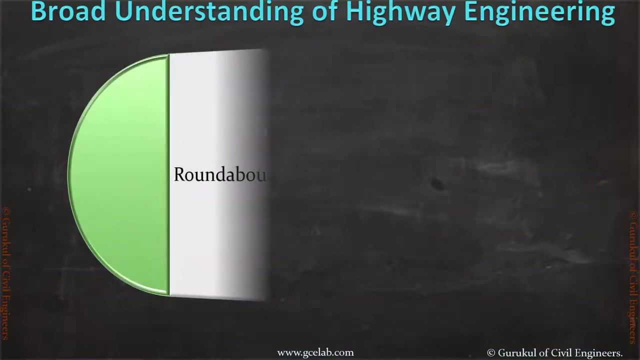 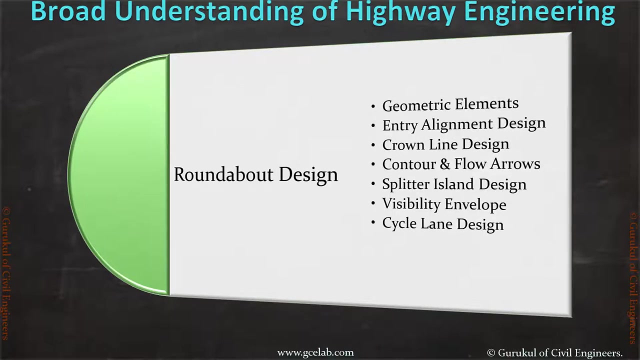 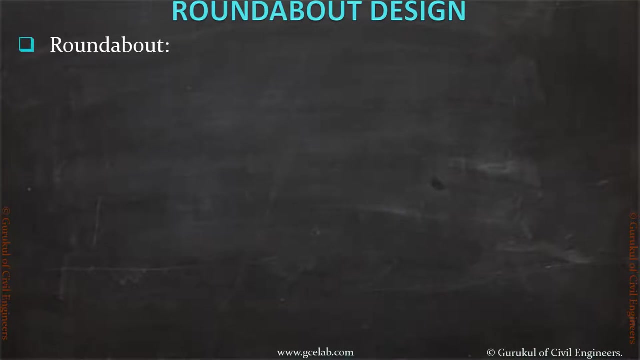 We will cover junction modeling and also the swept path analysis as shown in the pictures. Then we will cover roundabout design. Here we will cover geometric design, entry alignment design, crown line design, etc. Roundabout is one-way circular intersection where the traffic flows. 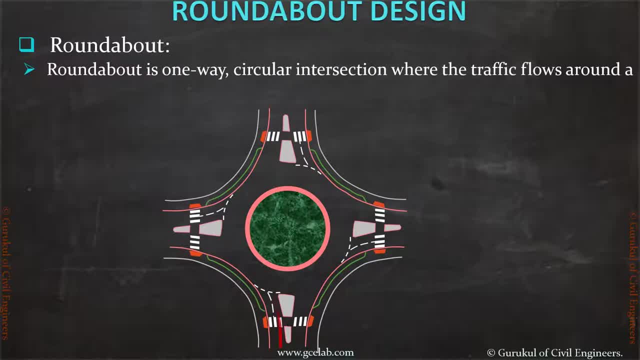 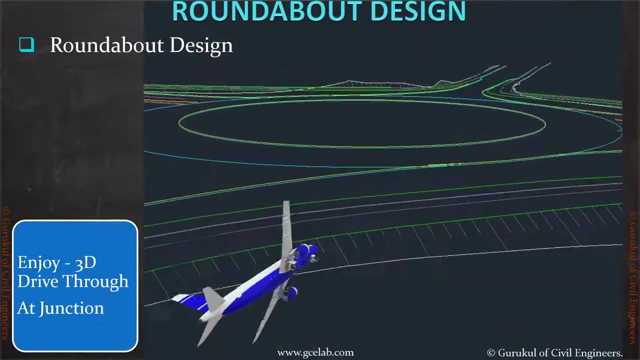 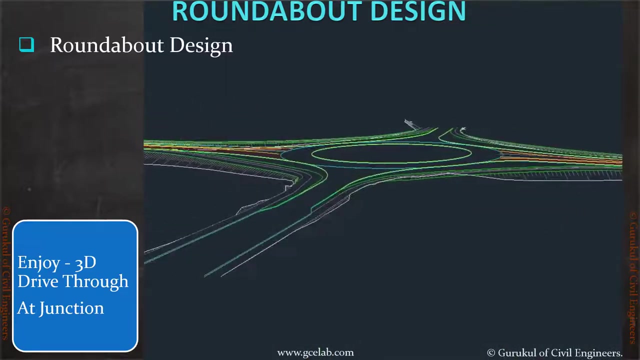 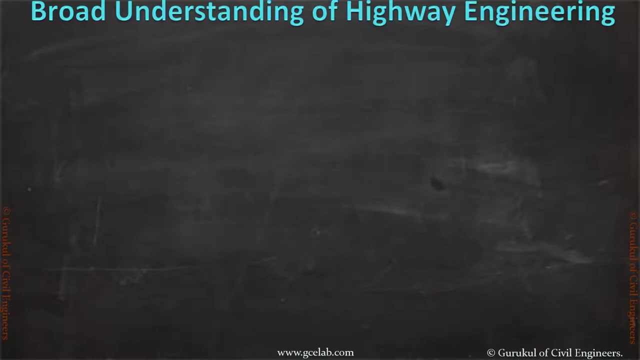 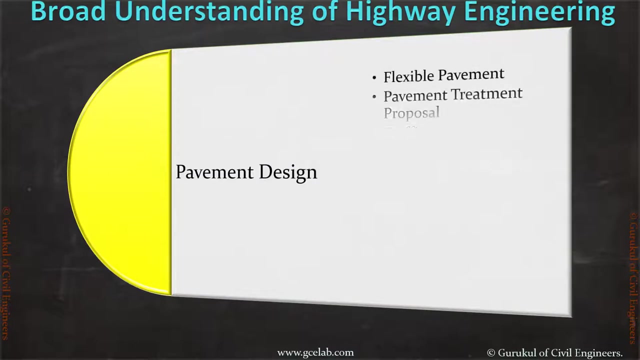 around the roundabout. Roundabout is one-way circular intersection where the traffic flows around a central island. We will cover complete process of pavement design, from traffic loading to pavement design and foundation design, etc. We will also discuss existing pavement improvement process and sub-grade improvement process.